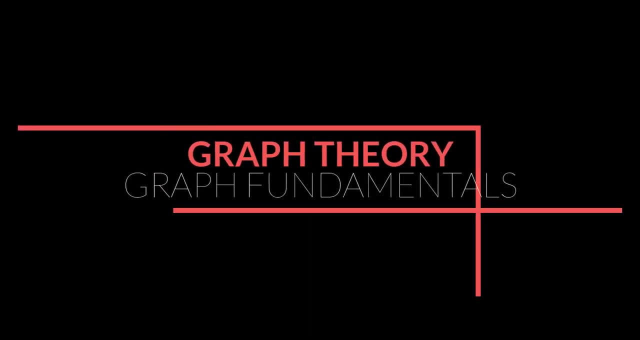 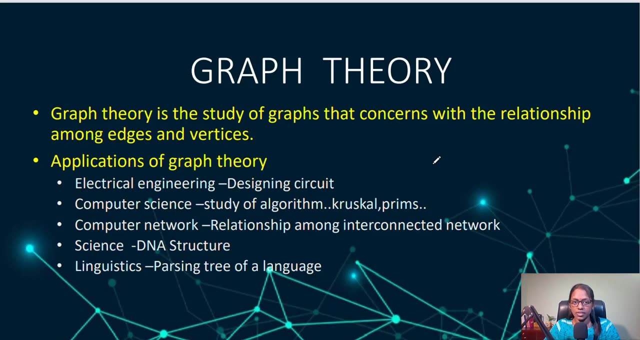 Hello friends, happy day to all. Today we are going to see graph theory. What is graph theory? Graph theory is the study of graph, that concern with the relationship among edges and vertices. So may I say to you, we are handling the edges and vertices of the graph. 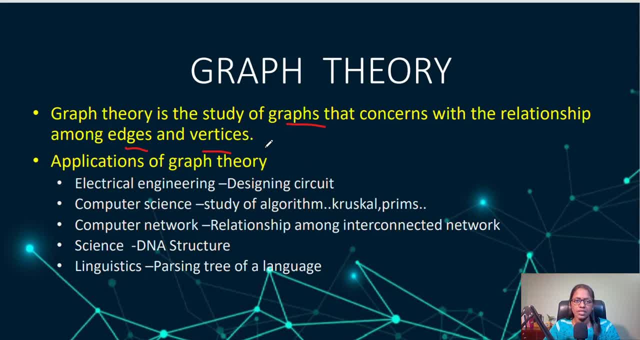 theory. So what are the applications of graph theory, Applications of what? wherever we are going to use this graph theory concept, it is called as an applications of graph theory. So where we are using in an electrical engineering, like designing a circuit, and in a computer, 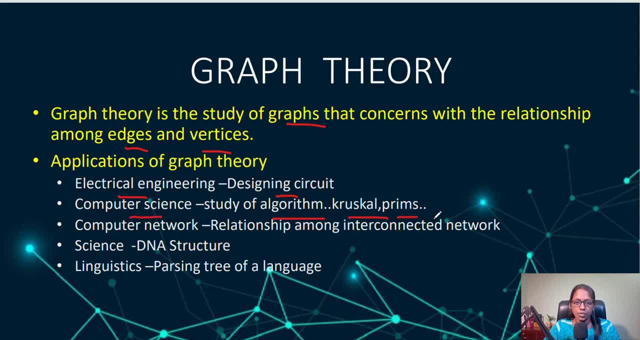 science like studying of algorithm, like Kruskal, Brum's algorithm and Kramling-Selfman algorithm and many more algorithms are there. It is based on the graph theory And in computer network relationship among interconnected network, So how it is relating with one network. 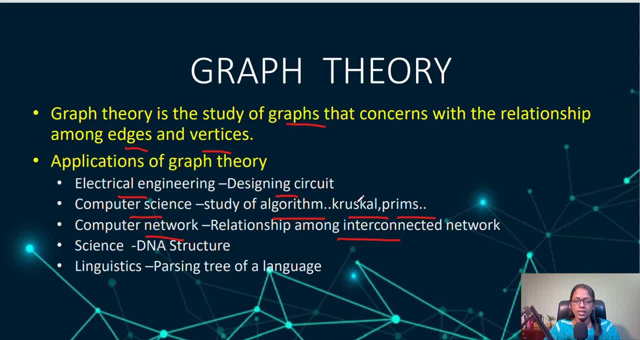 to another network. So in a computer network your relationship is identified using the graph theory, And in a science, in a science, we are studying about the DNA structure. So everything the DNA structure is similar like a graph, And in a linguistic we are doing the passing. 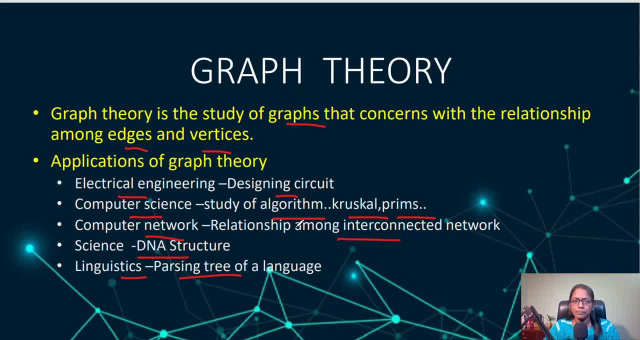 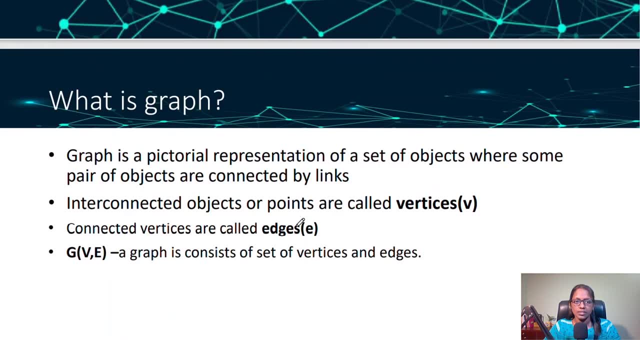 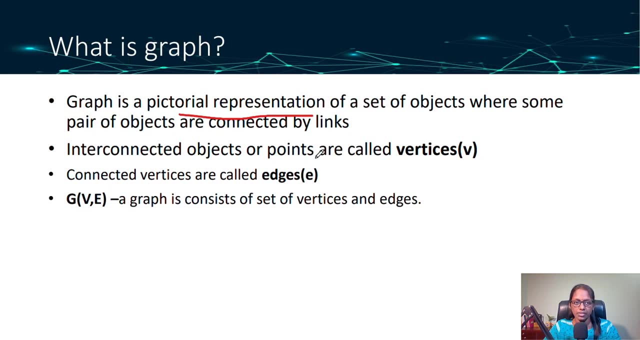 tree of a language. So this is the what, graph theory and the applications of graph theory. Yes, And the next one is: what is graph? Graph is a pictorial representation In a diagrammatically, we are representing a picture. 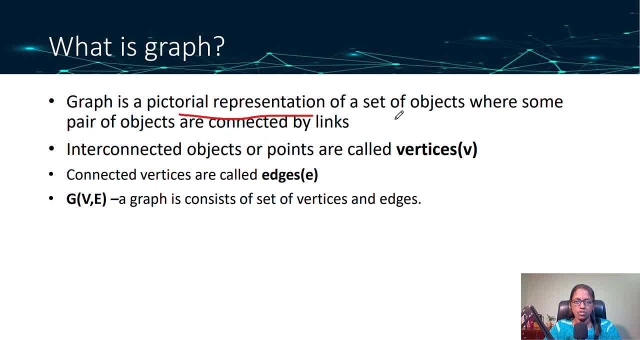 Okay. Graph is a pictorial representation, a picture representation of a set of objects where some pair of objects are connected by links- Okay. So consider: here this is A- Okay, And here this is B- Okay. A is an object and B is an object and C is an another object. 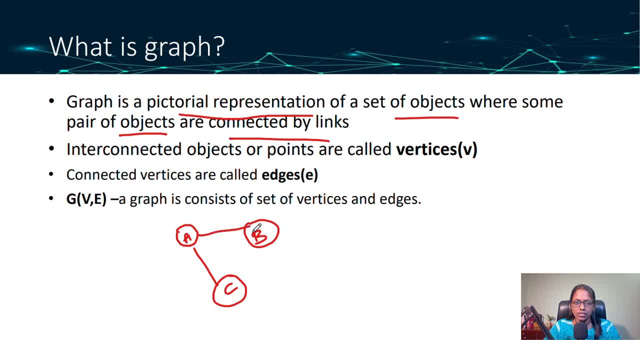 These objects are connected by the link. This is a line or link. So a graph is a pictorial representation of set of object. This is A, B, C is an object where some pair of objects are connected by links. Interconnected objects or points are called vertices. So this object, this is A and this B and this C is called as a vertices. 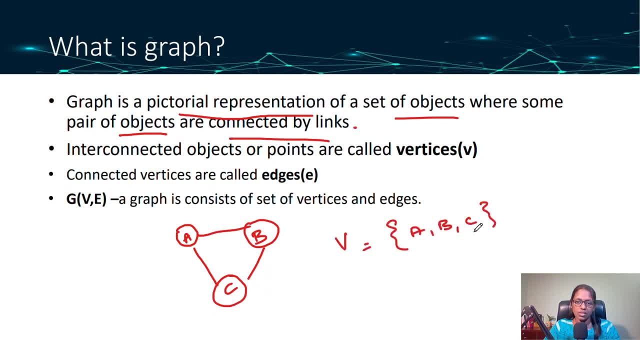 So what are the vertices here? A, B, C are vertices And the connected vertices are called edges. You can also name it as E1, this is E2 and E3. So how many edges are there in the group That is? 3 edges are there. So E1 and E2 and E3. So how many edges? 3 edges. 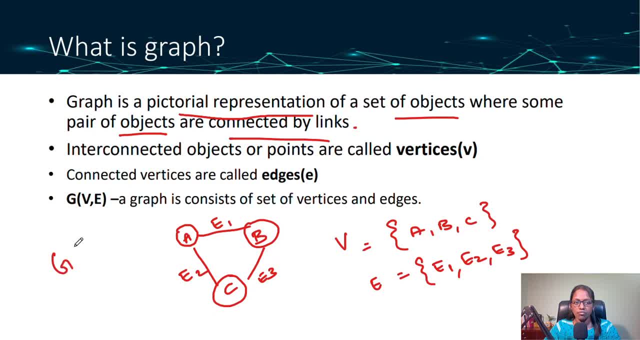 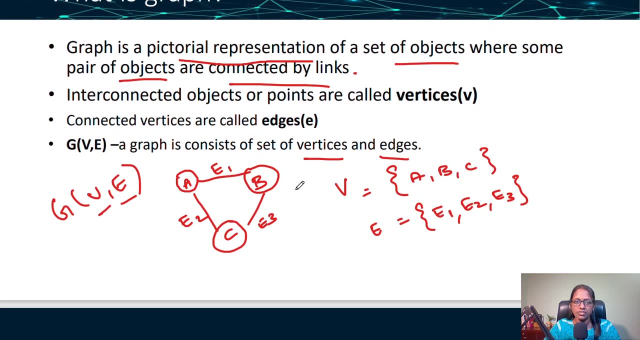 So the graph is consist of G of B, E, So it is called as G of B, E, The vertices and E is edges set. A graph is consist of set of vertices and edges, So this is a graph G. Here the vertices set is A, B, C and edges set is E1, E2 and E3.. 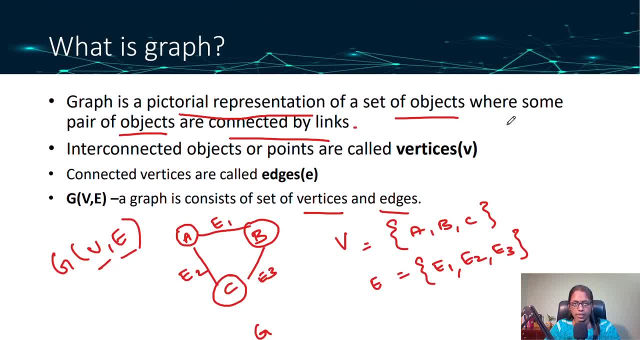 So this is what graph is. Graph is pictorial representation of a set of objects where some pair of objects are connected by link. Interconnected objects or points are called as a vertices And connected vertices are called as edges. And G of B, E is a representation of a graph which is nothing but V is a set of vertices set in a graph and E is set of edges in that particular graph. 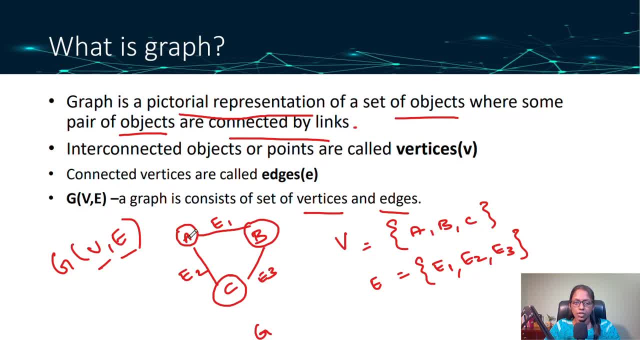 So, for example, in this graph G, what are the objects A, B and C? What are the edge set, E1, E2 and E3.. So V can be written as A, B, C and E is written as E. 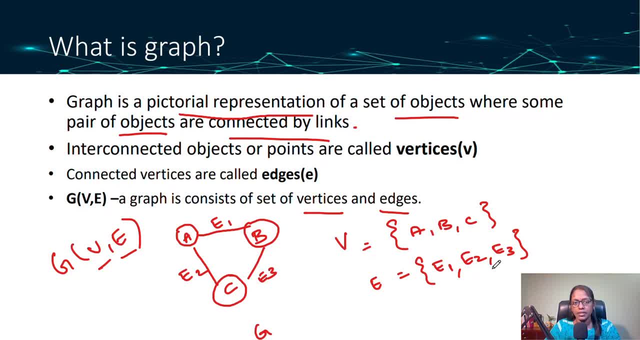 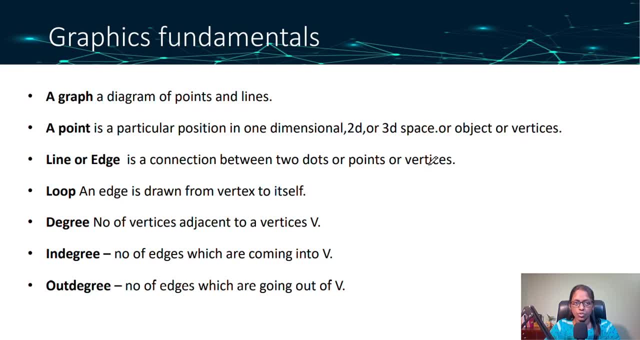 E1,, E2, E3.. Yes, Clear, Yes. So let me go to the next one. What is the set of words which we are using? Fundamentals, So graphic fundamentals, Normally. what are the words we are using and what are the meanings of that That we are going to see now. 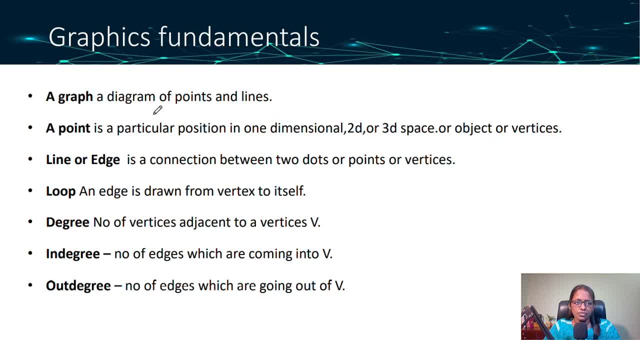 That is a graphics. fundamental is first one, a graph. A graph, a diagram, which consists of points and lines. Points is nothing but the object, Or this point, This points are connected with some lines, So this is normally call it as Graf. Okay, So this is normally call it as Graf. 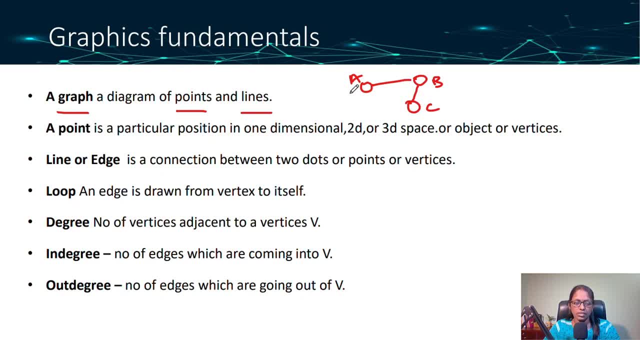 A graph is a diagram of points and lines. The next one is a point, is a particular position. Either it may be in 1 dimensional or 2 dimensional or 3 dimensional space. it can also called as an object or vertices. Okay, here the points were called as A, B, C. 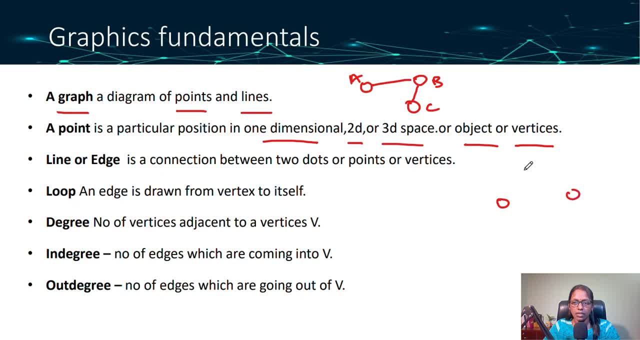 Okay, this may be in a one-dimensional, this may be in a two-dimensional, or this may be look like a three-dimensional. Okay, this is three-dimensional. So x and y is the dashes. So this is 3D space. Okay, 2D means only this. Okay, so this is called as a point or the position. 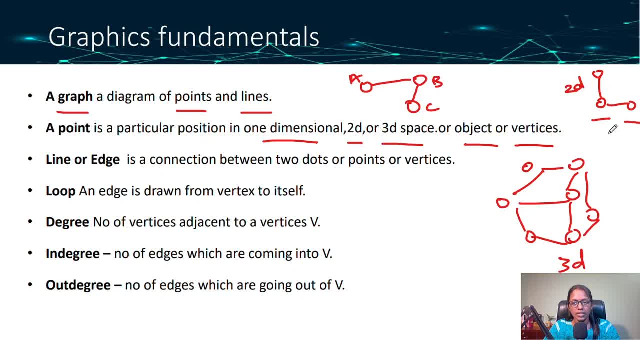 or this may be call it as an object, or this may be call it as a vertices. So everything is same. A point is a particular position in one-dimensional or two-dimensional, one-dimensional or two-dimensional or three-dimensional space, object or vertices. This is called as a point. The next one is called as a line or edge. So what? 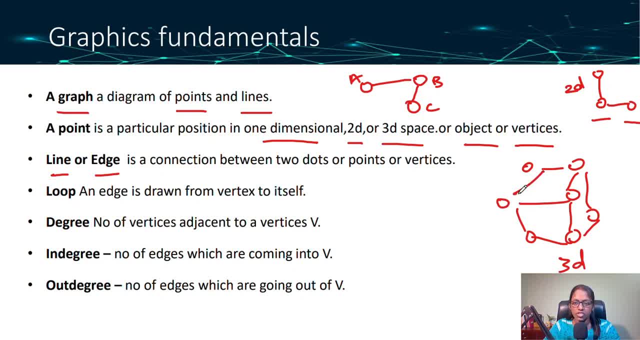 is line or edge, A line which is connection between the two dots. Here this is a two object which are connected between two dots or point or vertices. It is called as line or edge. So this is called as line or edge. So you know the meaning of what is graph, Points and lines, correct Point. 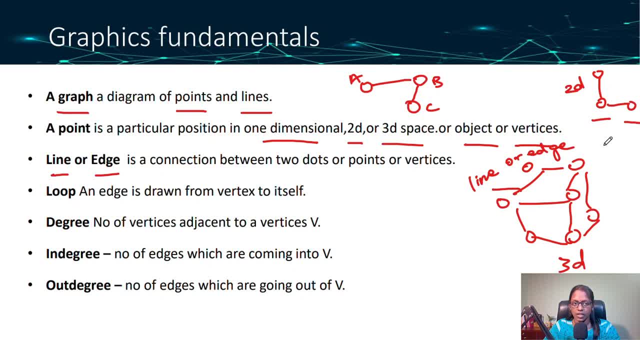 is. it may be in any object or vertices. It present either in a one-dimensional or two-dimensional or three-dimensional right. Yes, The next one is line or edge, which is a connection between the two dots or points or vertices. Yes, The next one is loop. What is loop? A loop? an edge is drawn. 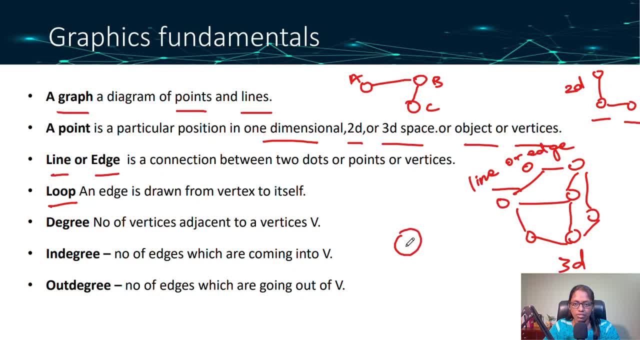 from the line or edge. So this is called as line or edge. So this is called as line or edge, So vertex to itself. So this is a vertex A, A vertex A, the edge is connected by itself. okay, Edge is. 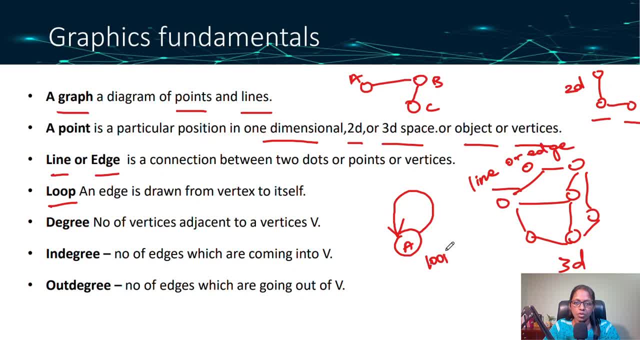 connected by itself. This one is called as loop. This one is called as a loop. An edge is drawn from vertex to itself. It is called as a loop. The next one is degree: Number of vertices adjacent to a vertex B. Number of vertices adjacent to a vertex B, For example. so A is a vertices. So what is the degree? 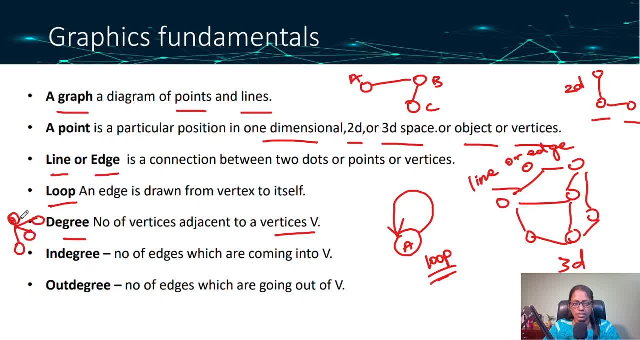 of A. So how many adjacent vertices That is from A, how many lines are connected? One, two, three, okay, So three, So three is the degree of that vertex A. Three is the degree of vertex A okay. 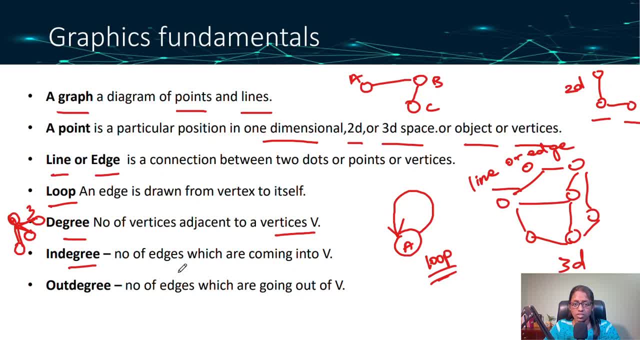 The next one is in degree. In degree means number of edges which are coming into V. So V is a vertices, Okay, V is the vertice, And number of N degrees coming. Okay, That is in a direction. So here one direction. 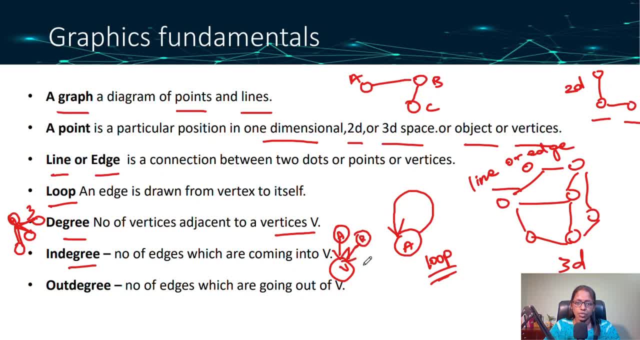 is there. If I put two direction, then degree is two. Okay, So the in degree is two. Now, number of edges which are coming into B Out degree is number of edges which are going out of V. So from V, how many edges are going out? 2. So it may be. 3. So, whatever it is, 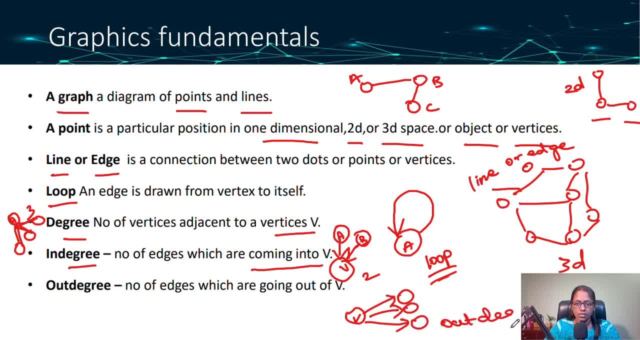 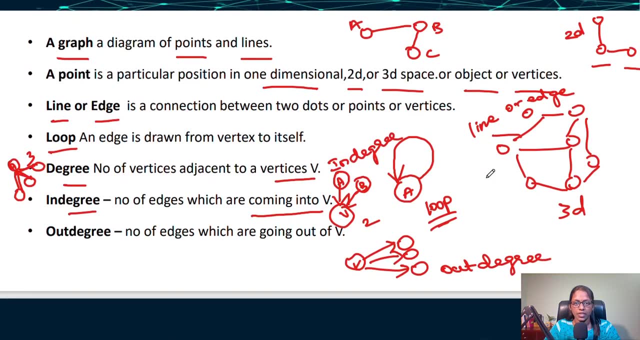 So this is called as out degree. So this is called as an out degree and this is called as an in degree. So now you clear what is graph, a point, a line of edge and loop and degree. What is in degree and what is out degree. Yes, The next one is isolated vertex. 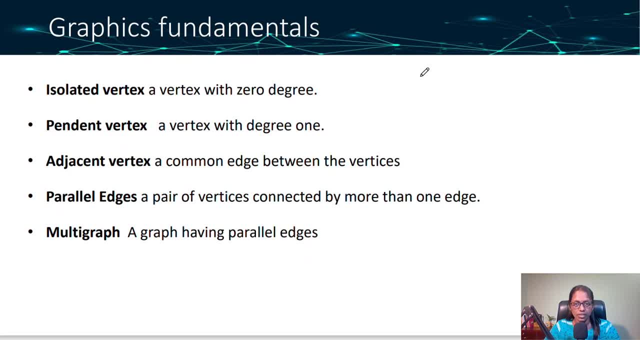 Isolated vertex means a vertex with 0 degree, So there is no degree for this vertex. Okay, Consider this is this one is an isolated vertex. This is isolated vertex. The next one is pendant vertex, A vertex with degree 1, which is called as a pendant. 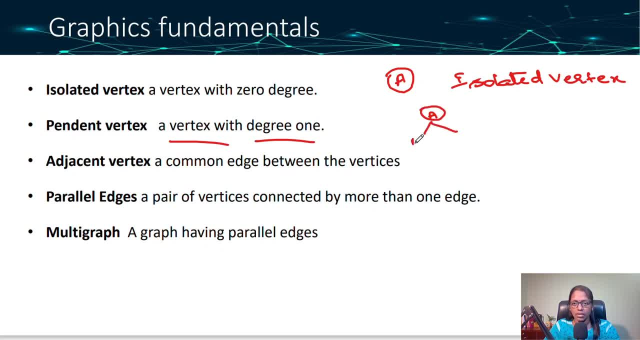 For example, A is there and B, C is there. So what is the degree of B? 1. What is the degree of C? 1. What is the degree of A? It is 2. There are 2 lines right, 2 neighboring. 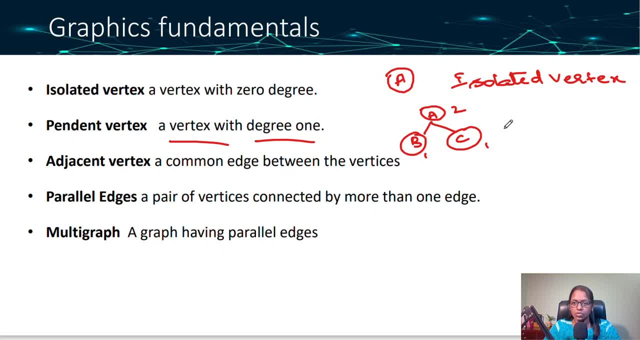 nodes, So a vertex with degree 1.. So B, C are called pendant vertex. B and C are called pendant vertex. The next one is adjacent vertex. Adjacent vertex is a common edge between the vertices. So what are the adjacent vertices? is A to B, So this is an adjacent vertex, So A's adjacent. 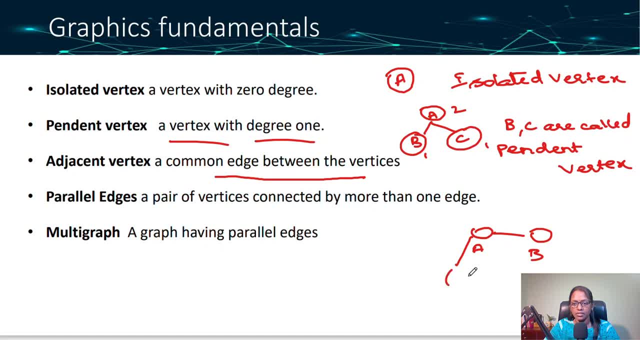 vertex is B and A's adjacent vertex is C. So what is the adjacent vertex is nothing but a neighboring vertex. Neighboring means normally we call it as a neighboring means the next to your out Right, The next person, the next house. Okay, So A neighbor is B and C. So B and C are called. 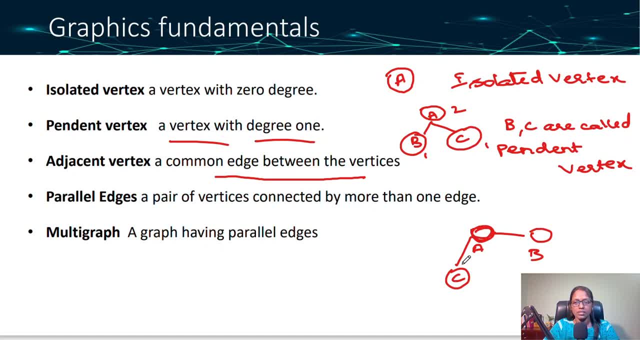 as an adjacent vertex of A, B and C are called as an adjacent vertex to A. The next one is parallel edges, Parallel pair of vertices connected by more than one edge, So a pair of vertex. So this is A and this is B. Okay, This is adjacent vertex. I don't. This is 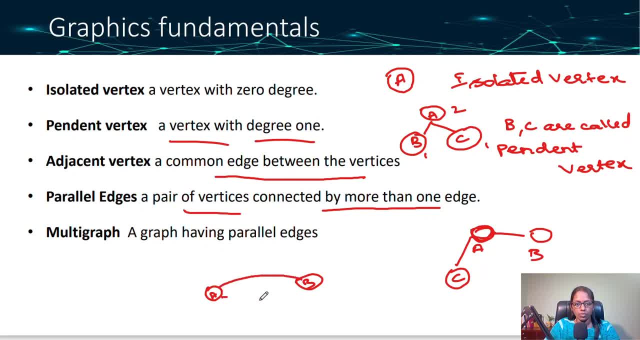 A and this is parallel edges. So this is one edge and this is another edge, Right? So this is called E1 and this is E2.. This- E1 and E2- are a pair of vertices. Okay, So this is called parallel edges. This is called parallel edge- A pair of vertices connected by more than 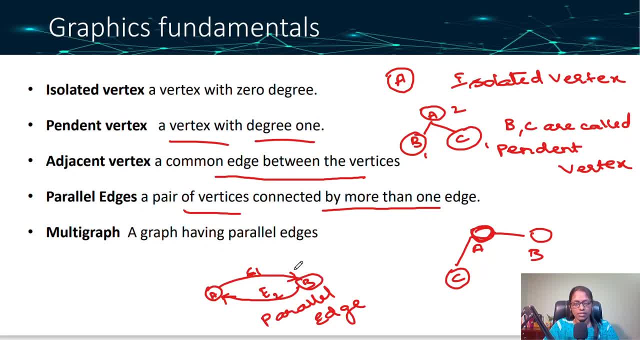 one edge. So this is one. A vertex and B vertices are connected by two edges and also have an equal and in a same way. This is called parallel Right. So parallel edges: A pair of vertices connected by more than one edge. The same vertices connected by more than one edge, which. 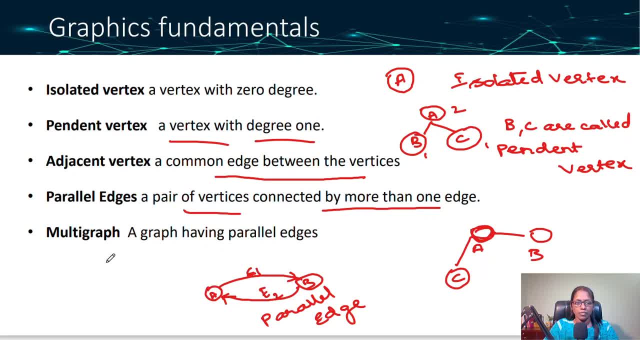 is called as a parallel edges, So multi graph. Multi graph means a graph having parallel edges, So when consisting of: So this is a multi graph, So this is called as an Each, this graph having parallel edges, also having many edges, So this graph is called.